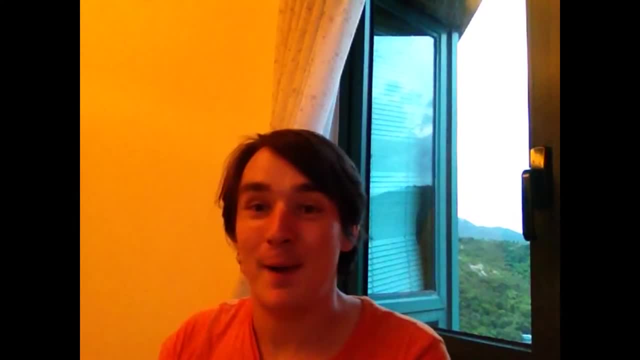 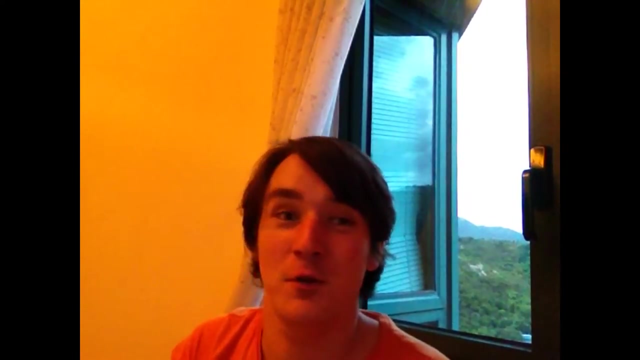 But anyway. so let's start talking about topology. What is topology? It's been defined as something some people call it rubber-sheet geometry. This is a very rough way of defining topology. A more kind of long-winded definition would be: it is the study of properties of shapes which are preserved by continuous deformations. 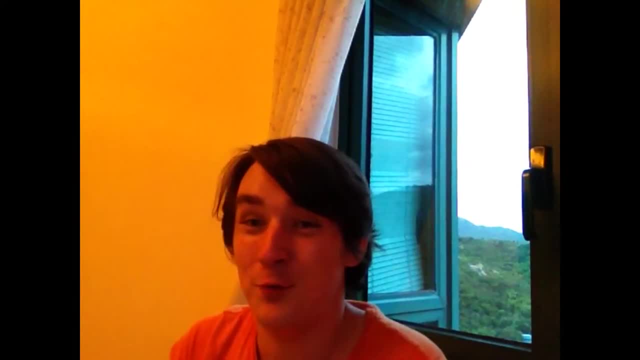 The second one sounds a little bit hard to swallow, so let's go with the first one. Let's think about it as rubber-sheet geometry. So for the first couple of lessons, I want to talk about some surfaces. okay, So here's an example of a surface. essentially, 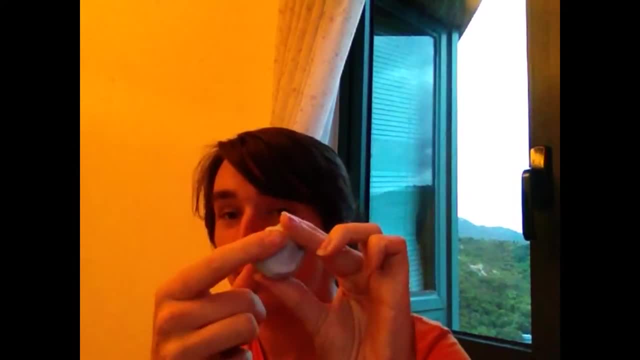 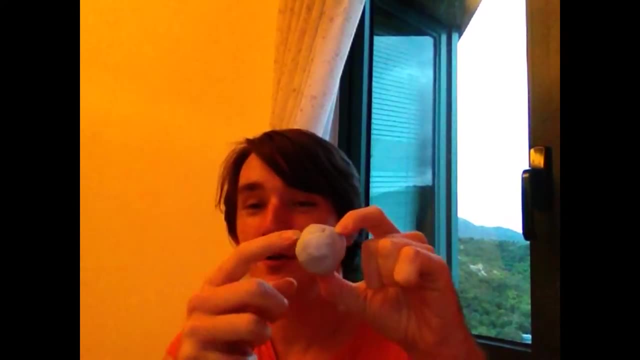 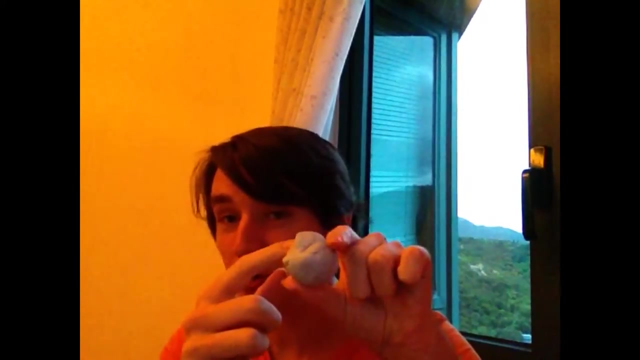 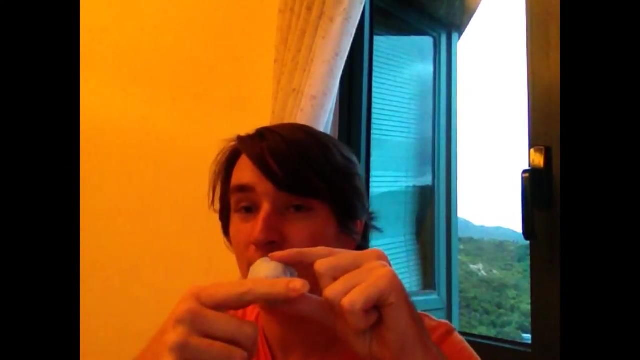 The outside of this ball. So you can think of this as a kind of two-dimensional surface. This is like a little model of planet Earth, right? You can imagine a little creature. It could walk around on the outside of this surface. And it's two-dimensional because this creature can go in two different directions which are kind of at right angles to each other. 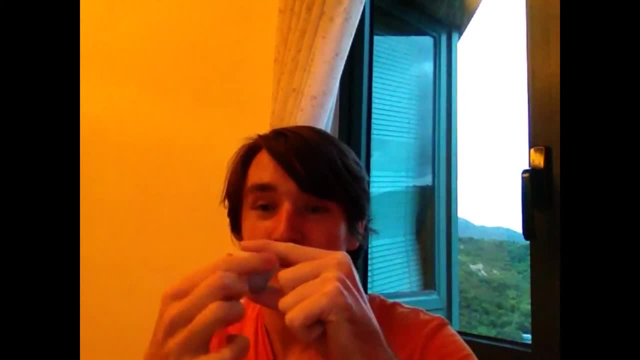 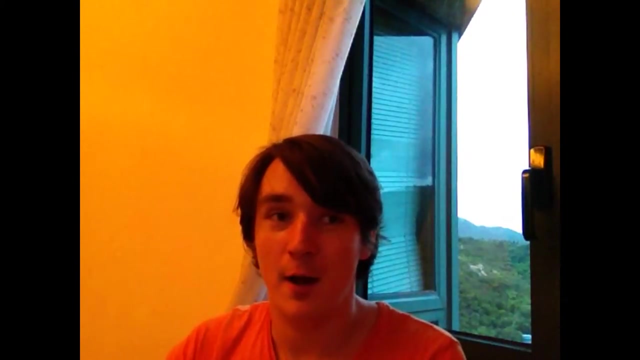 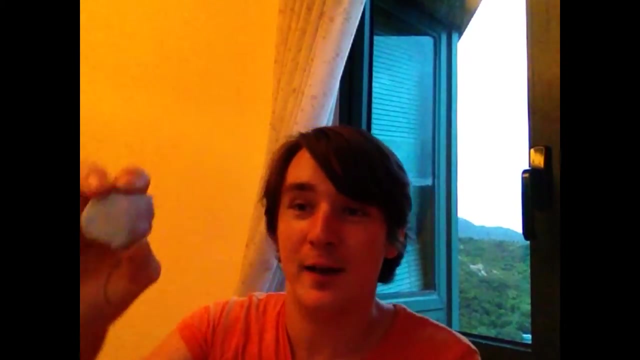 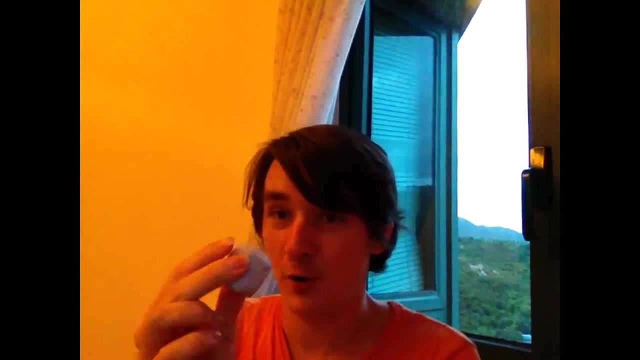 Okay, So this is one kind of surface, And in topology we're interested in surfaces. So another kind of surface would be a cube. Okay, So let's make this blue tack a little more cube-like now. The thing is, though, in topology the cube and the ball are actually the same from a topological viewpoint. 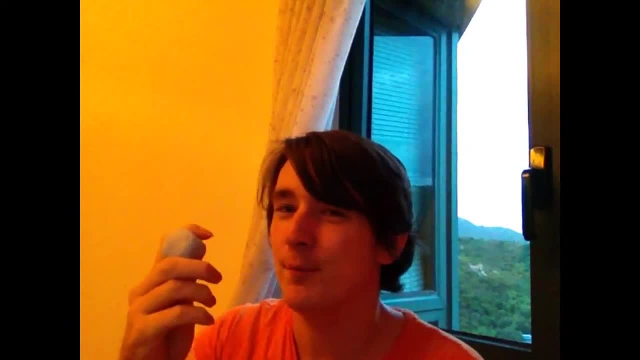 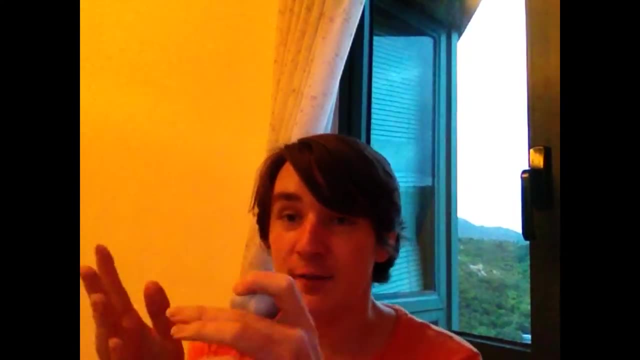 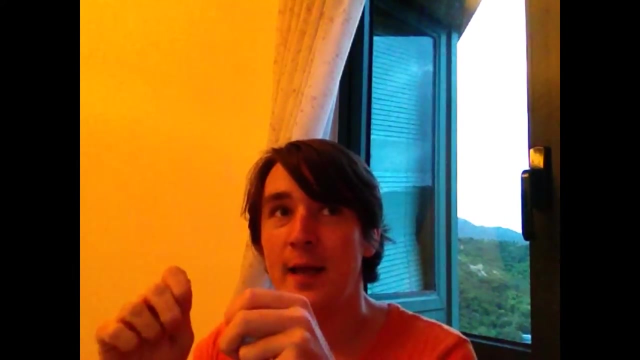 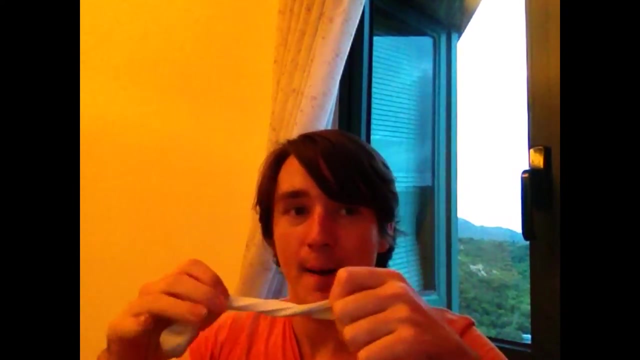 What do I mean? Well, what I mean is whenever you can continuously deform one shape into another. topologically speaking, they are the same, So let me try and say this a bit more rigorously. Essentially, whenever you can deform an object by doing stretching and twisting and bending. 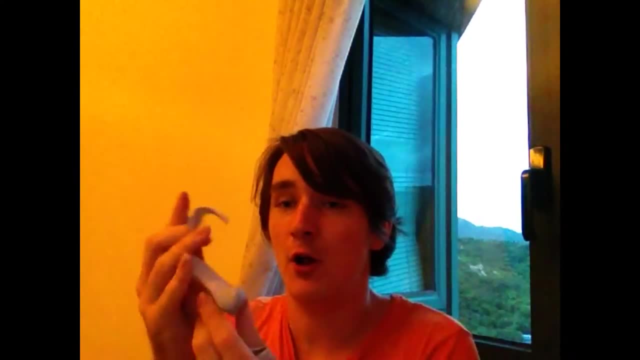 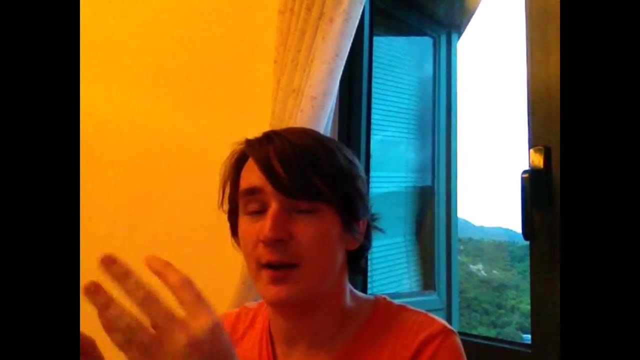 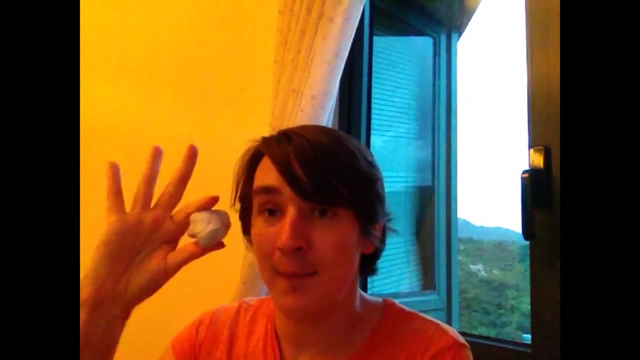 but not breaking and not sticking. whenever you can deform an object like that into another object, those two things are essentially considered the same. So, for example, I have this ball-shaped surface here. Okay, But I'm imagining it's made out of a very malleable thing like rubber. 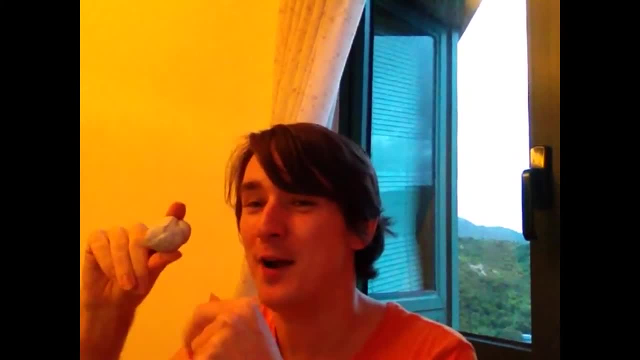 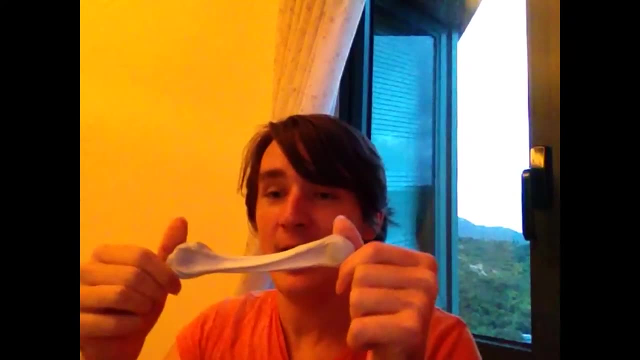 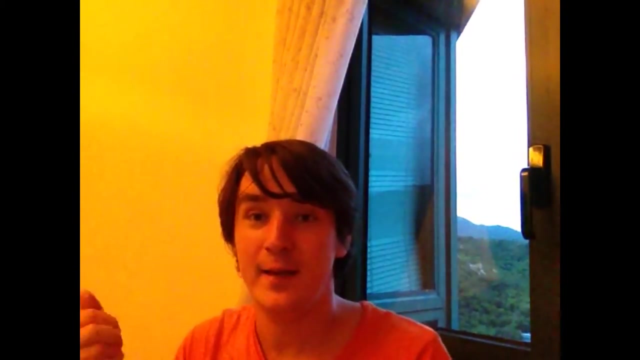 Actually I don't have to imagine, Because it's made out of blue tack, right, So I can do a continuous deformation of it, I can stretch it out, And it's still topologically equivalent to a sphere. So in topology we are allowed to make these continuous deformations. 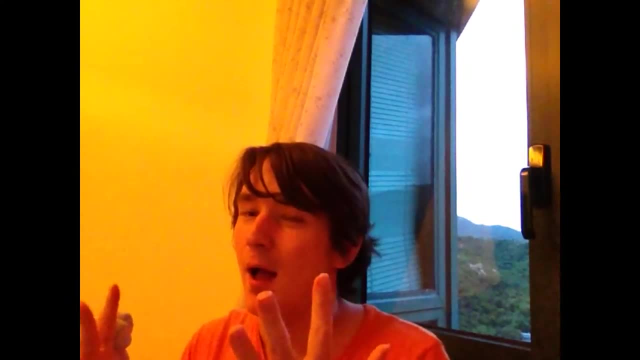 And so really the magic of topology is that you forget about certain details. You see this in different areas of mathematics. that kind of by half-closing your eyes and by forgetting about differences between objects, you can get a kind of higher viewpoint. 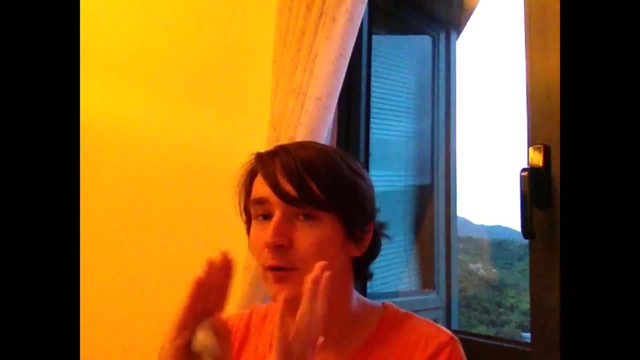 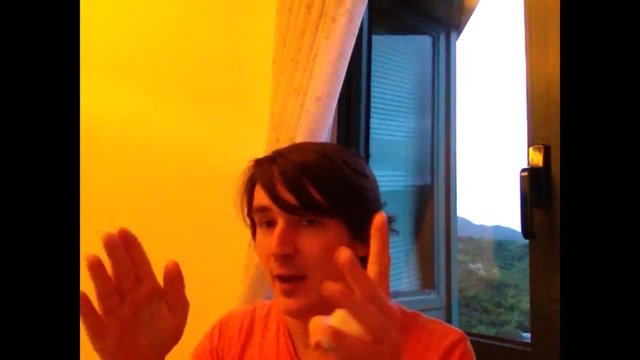 Like in topology, we disregard lots of details about shapes. For example, we're not interested in the distances and the corners and things of the cube. In our view, a cube is just about the same as a ball. Well, you might think then. 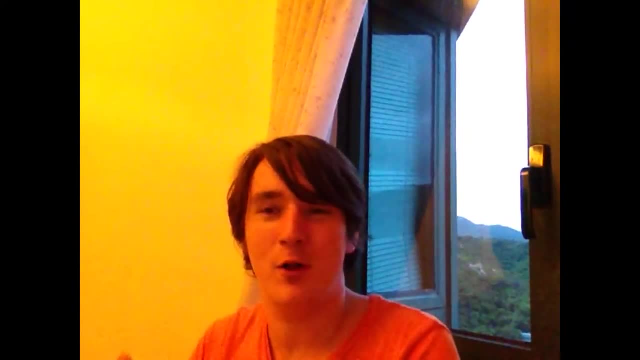 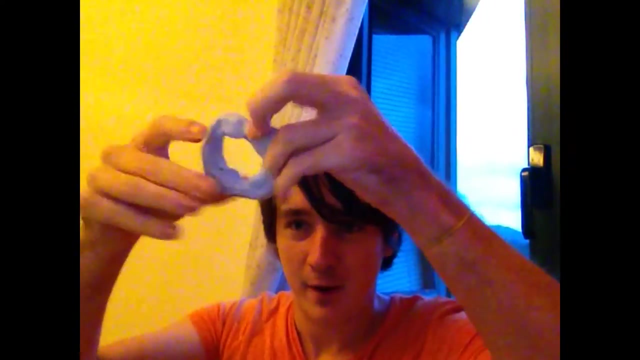 if everything's the same in topology, then what's the point in studying it? Well, the thing is that everything is not the same, Because some surfaces are topologically different to other surfaces. So let me show you a simple example. This is a torus, okay. 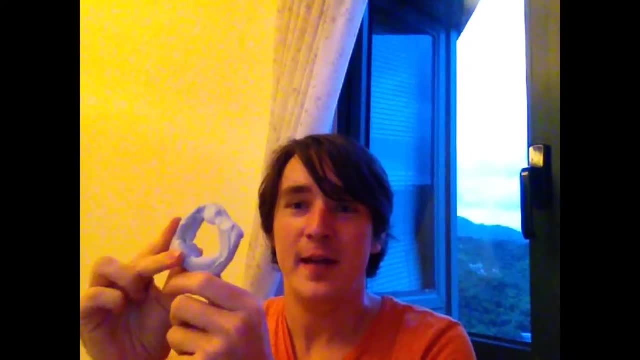 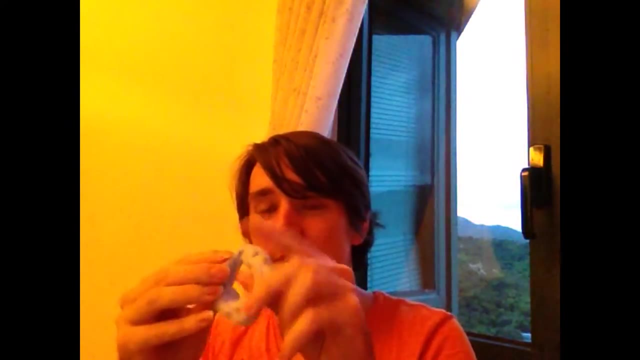 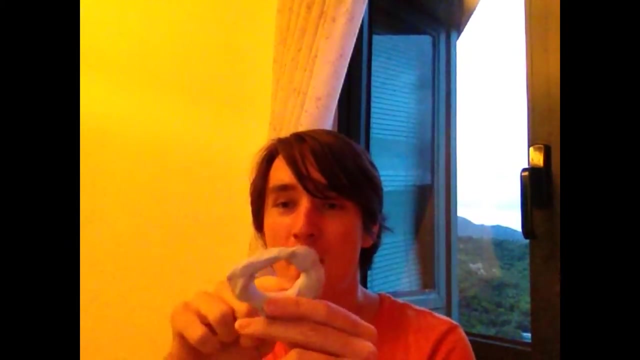 It's basically the kind of shape of the inside of a tire or the shape of a doughnut, So it's a two-dimensional surface with a hole in it And again you can imagine that you're a little creature walking around on this surface. 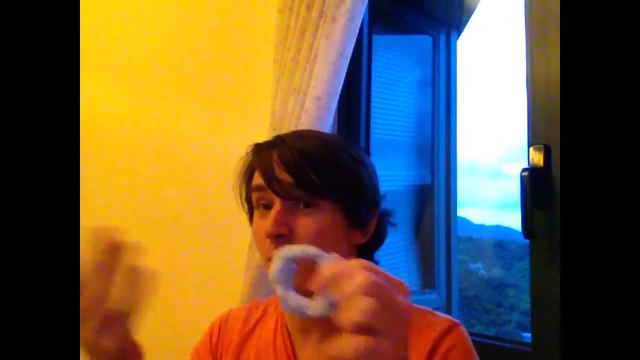 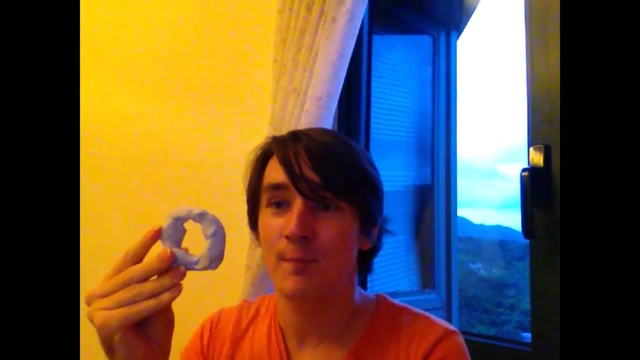 And you could walk all around it. And how would you know if you were walking around on a torus? It's a good question. Anyway, I claim that this torus is not topologically equivalent to a sphere And hopefully you can see that right. 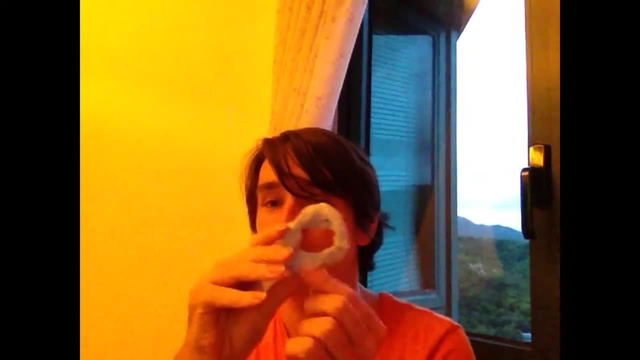 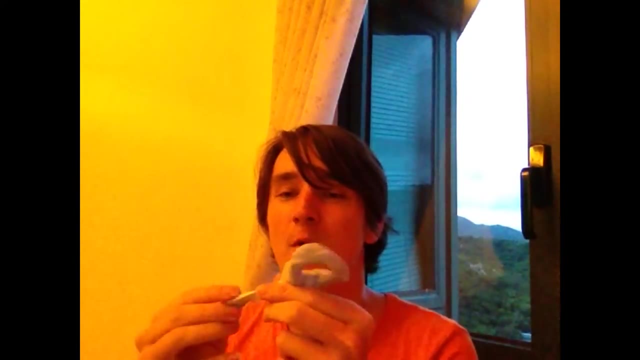 Because we can deform this thing quite a lot. I mean, we can crush it, We can pull things out, We can twist them, We can do all kinds of things, But we're not allowed to stick any two points together that weren't initially close to each other. 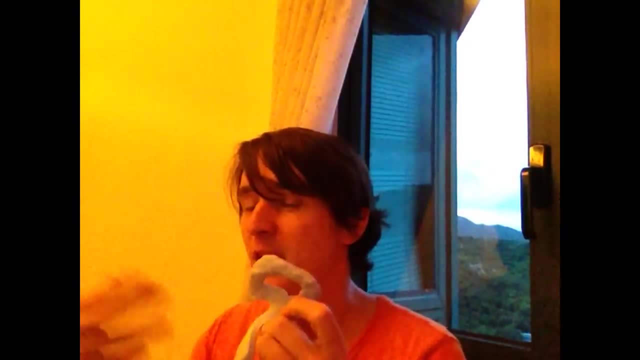 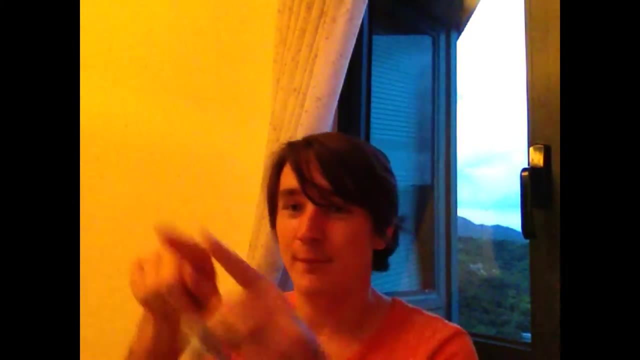 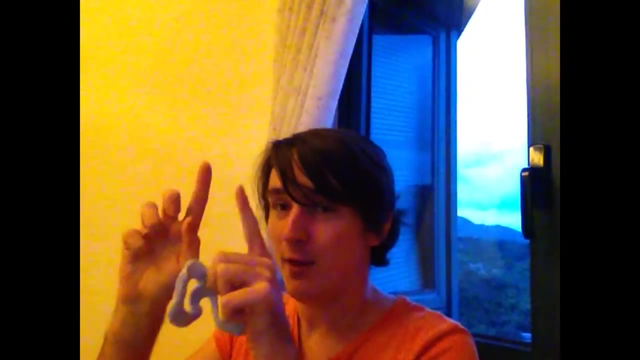 Basically, the kind of operations we're allowed to do are like this: If two points were close before we do something, then they have to be close after we do something, And if two points were far away before we do something, then they have to be far away after we do something. 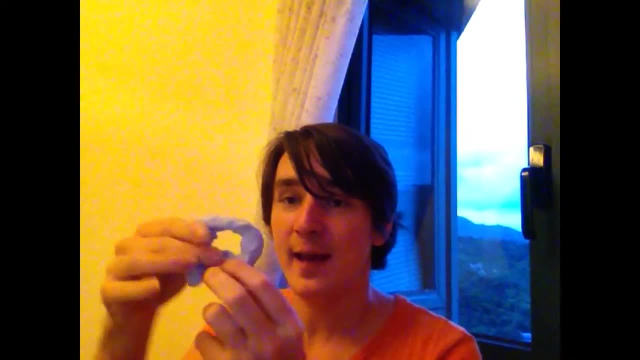 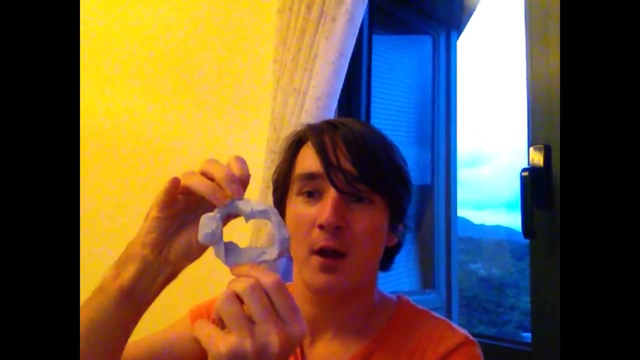 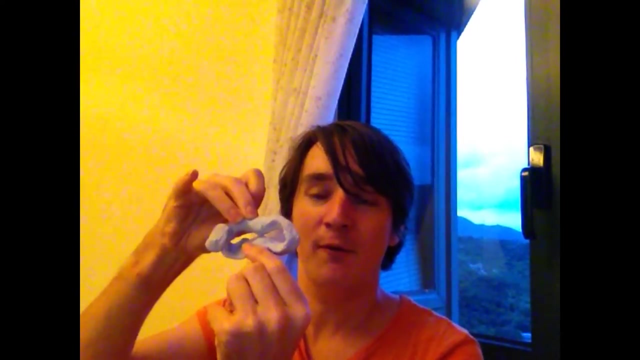 And that's why we're not allowed to do any sticking. So we're not allowed to sort of stick like this, because we had a point up here and a point down here which were far away from each other, And then suddenly we've changed the topology of the shape. 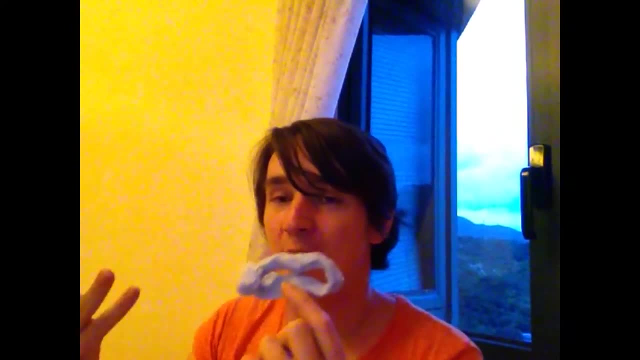 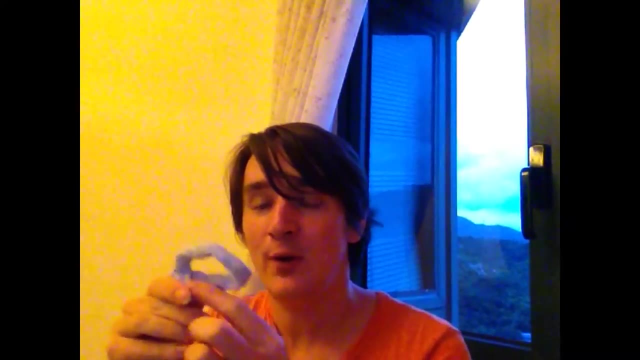 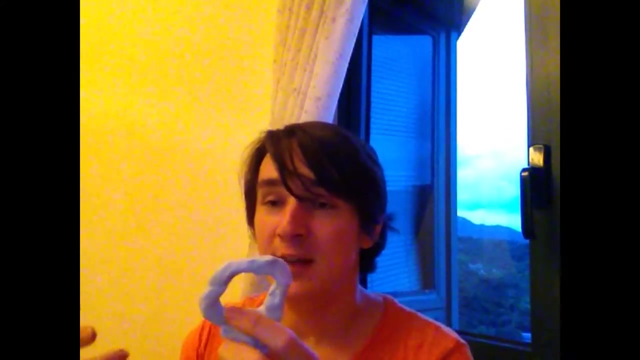 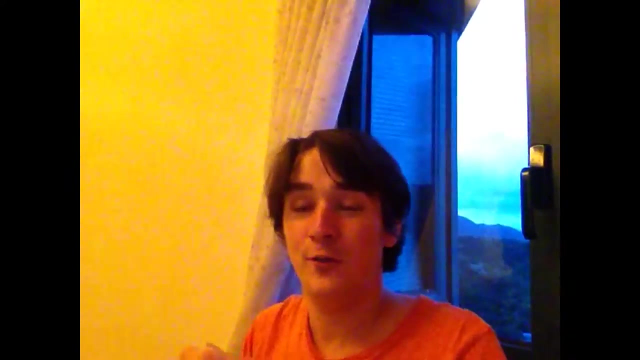 by making these points close. So that's an illegal operation. So all we're allowed to do is bending and twisting and things, And hopefully you can see that this torus is topologically different to a sphere, So it's sometimes said quite jokingly. 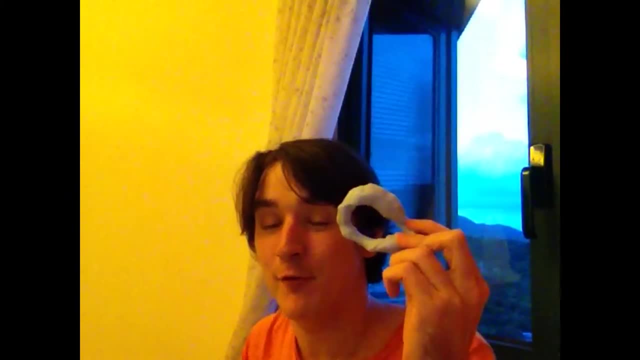 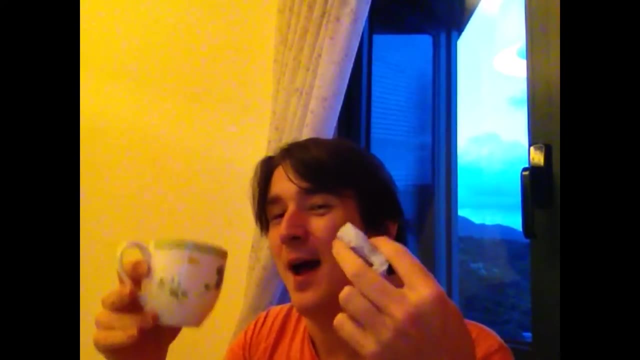 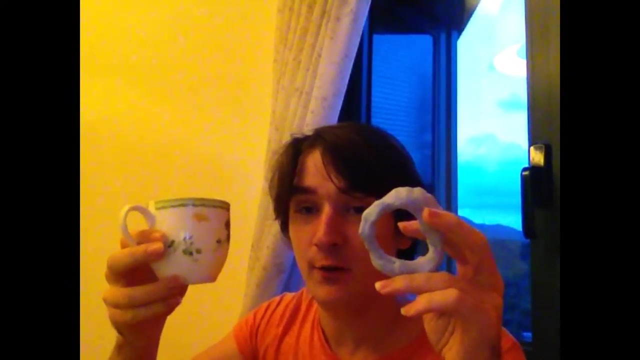 that a topologist is somebody who can't tell the difference between a doughnut and a coffee cup, And the reason they say that is because these two objects are essentially topologically equivalent. In other words, if we imagine that this was made out of rubber, 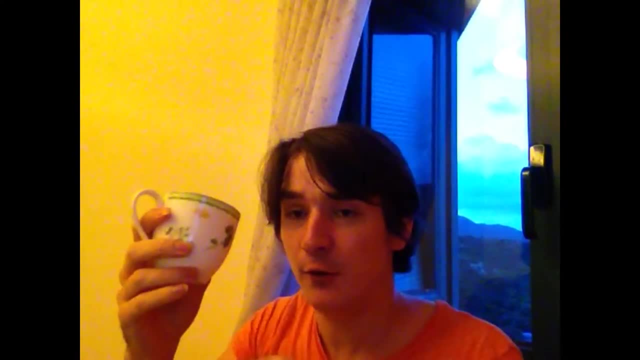 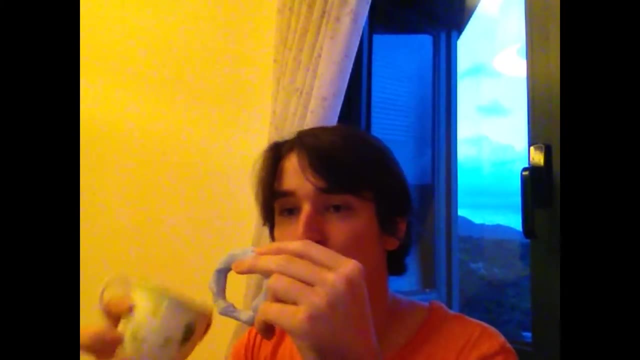 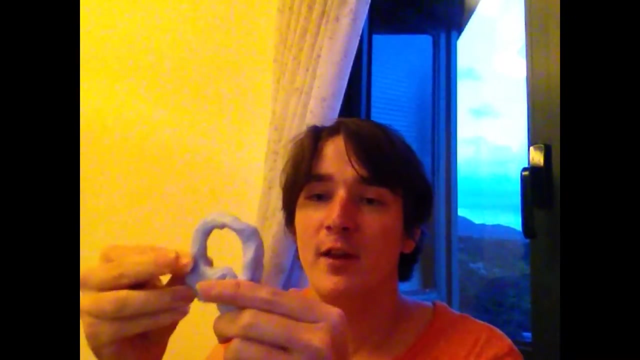 or something really malleable. we could continuously deform it into this Or, equivalently, we could change this to make it look like that. Well, let me have a go at doing this in front of you. So let's try and continuously deform this into something. 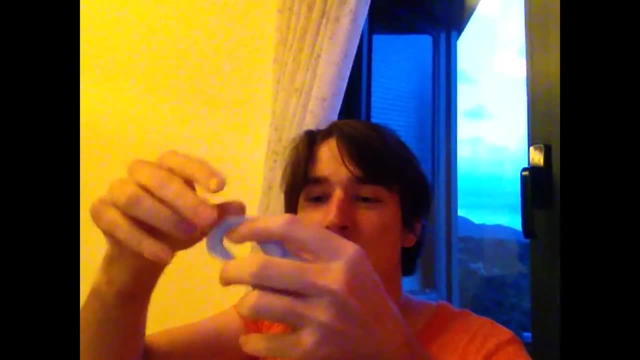 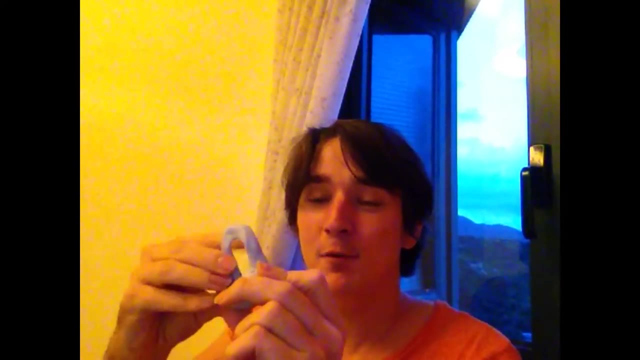 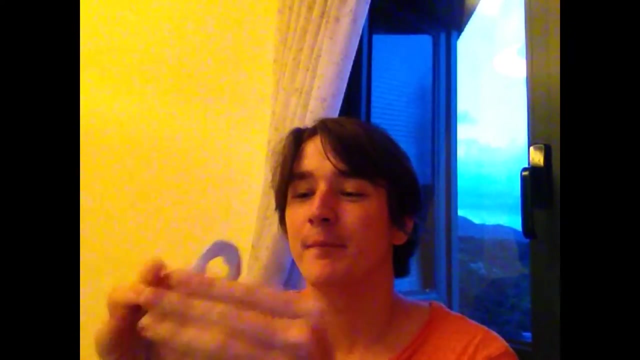 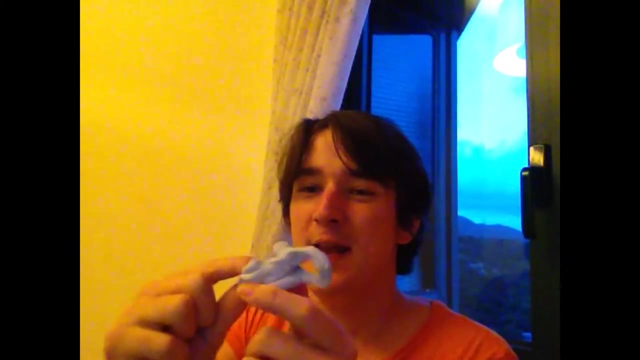 that looks vaguely like a teacup. OK, It won't be that convincing because I don't really have enough blue tack to make a proper teacup, but let's give it a try. Well, there we have it, So you could put your hot beverage in here. 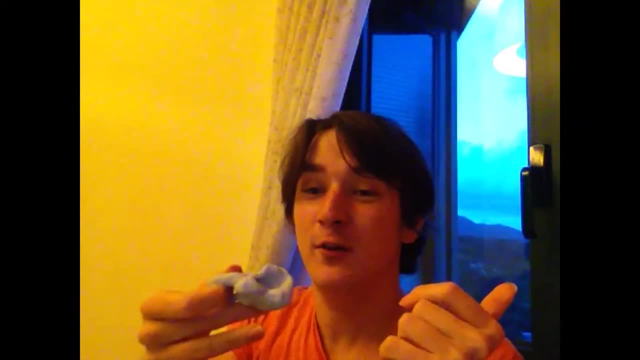 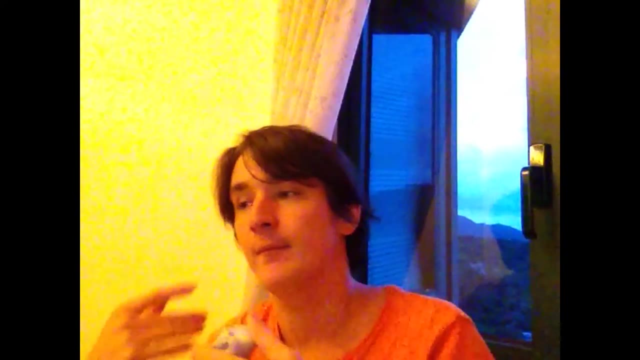 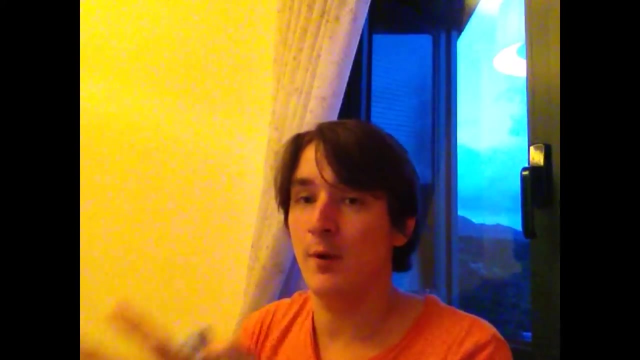 And this is your handle, And you could drink your tea out of this. So yes, you can see that these two objects are topologically equivalent to each other. You can look at all kinds of objects around you and think about this: Do they correspond to an object with one hole in them? 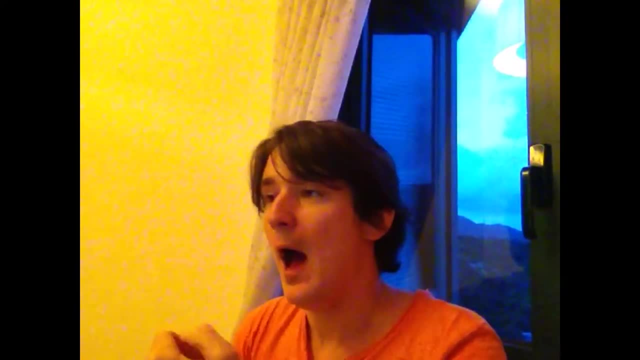 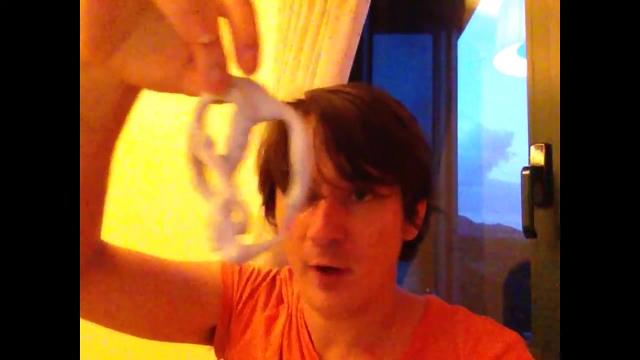 or two holes, or three holes, Et cetera. So what I'd like to leave you with is a fairly intriguing puzzle, So I'm going to show you this puzzle now. OK, So I'd like you to take a look at this object. 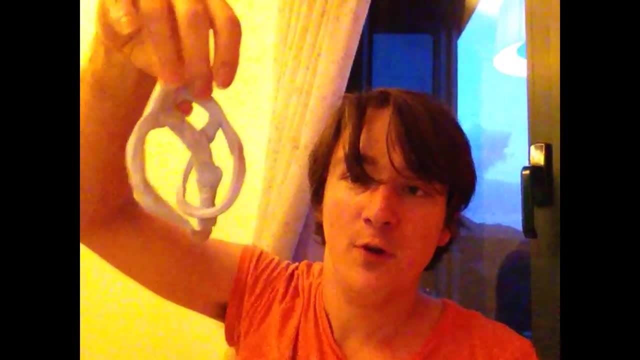 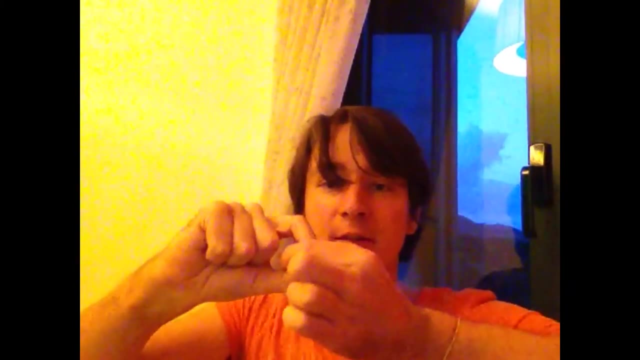 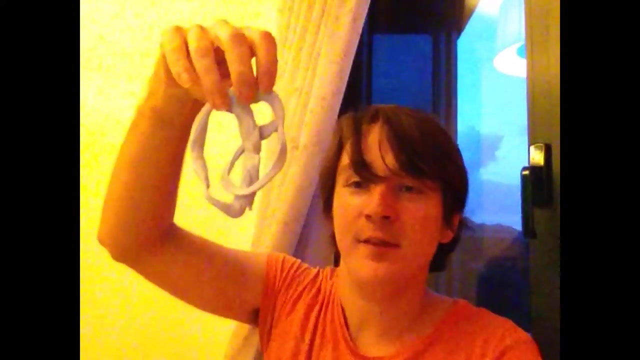 Essentially, this consists of two interlocking rings. I mean, if I link my fingers together like this, I'm sort of topologically equivalent to a shape like this. It has these two rings which will correspond to my fingers being interlinked. 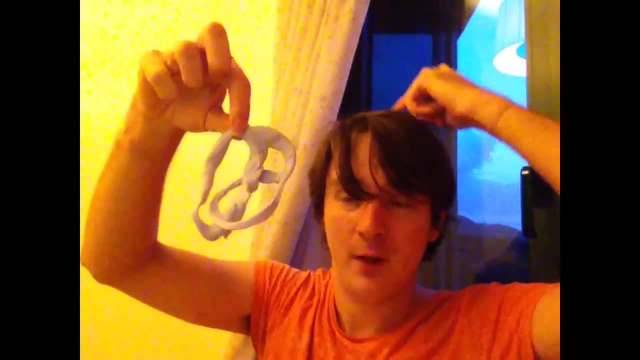 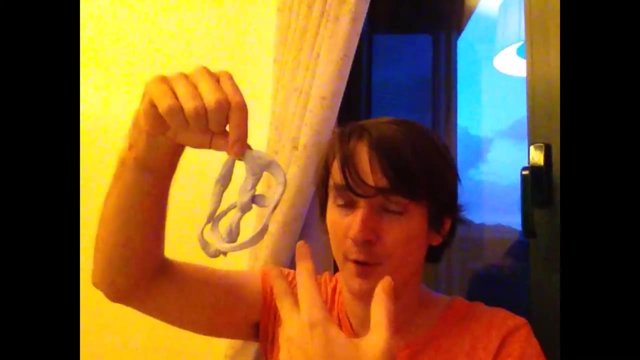 connected to a solid part. So another way you could think of this, you could think of this as a torus with two holes, but one of those holes is kind of linked in with the other one. OK, So you see this object. 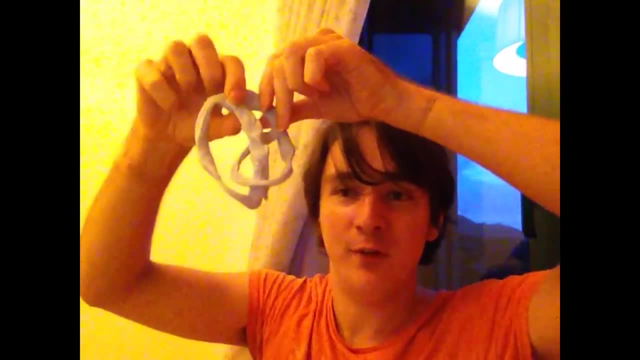 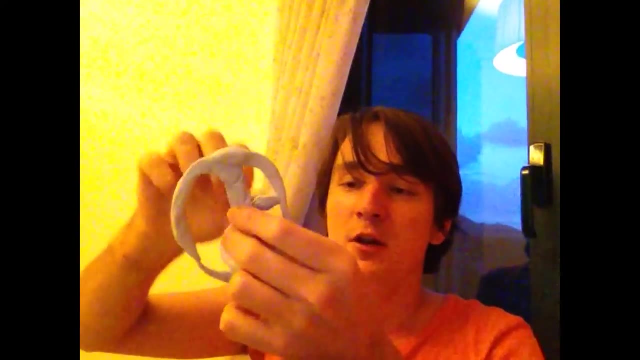 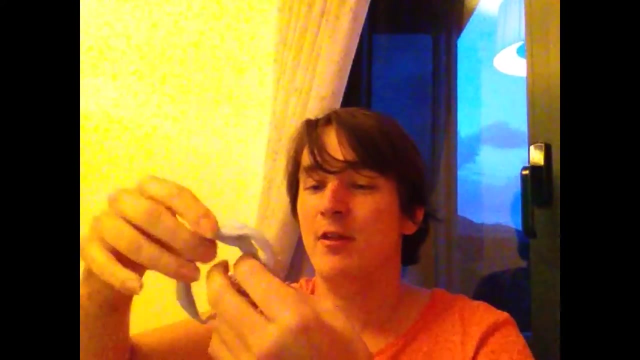 Take a good look at it. Think about it as a topological object. So think about all the things you could do with this. I mean, you can mess around with it, You can bend it and twist it and crush pieces together and all sorts of operations. 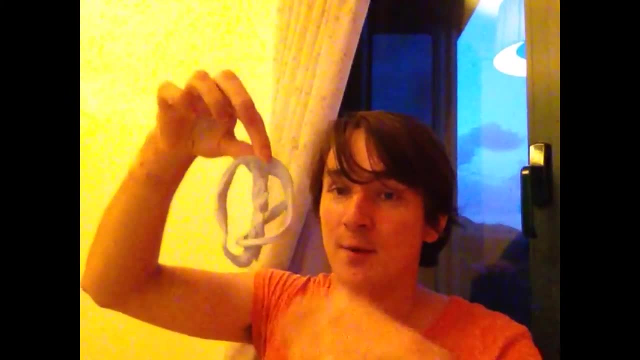 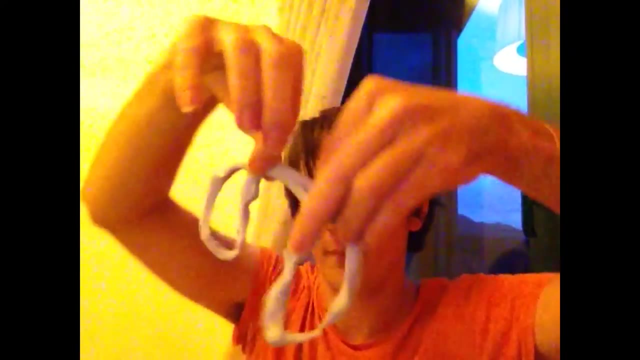 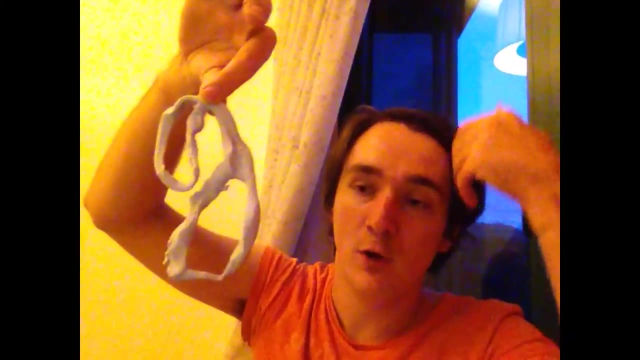 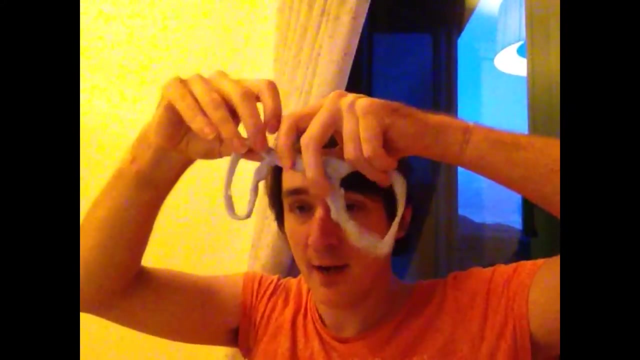 So the problem I'm going to set to you is to transform this object here into this object here. Now you're supposed to do this, obeying the laws of topology. So you're only allowed to do bending and stretching and twisting. You're not allowed to do any tearing or cutting. 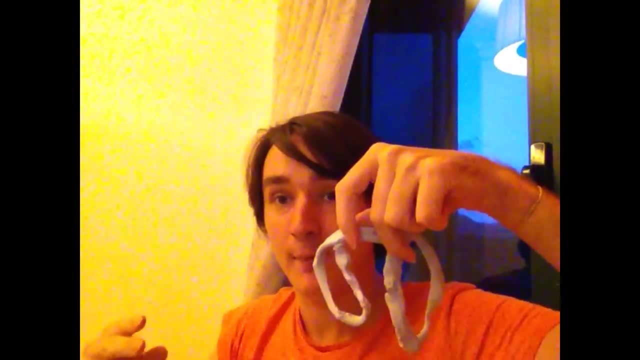 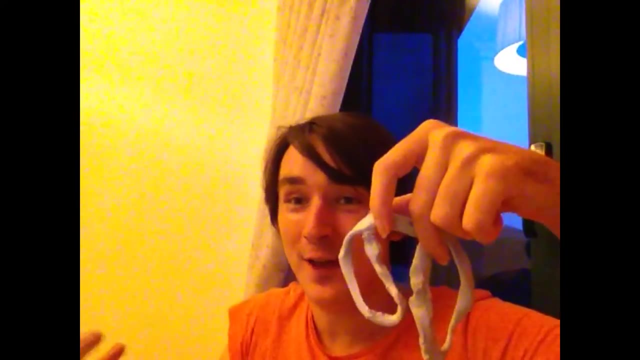 And, importantly, you're not allowed to do any gluing. OK, It's actually kind of hard to avoid doing gluing when you're working with Blu-Tack, since it so naturally sticks to itself, But you're not supposed to do any gluing. 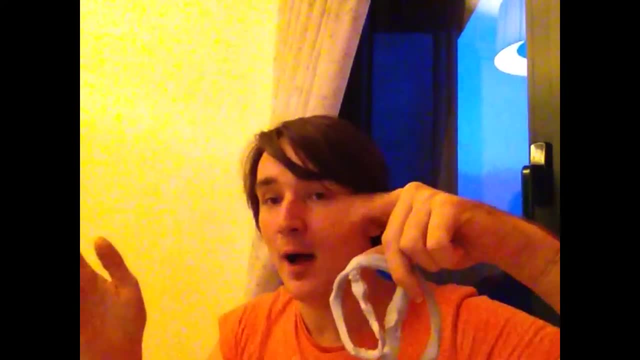 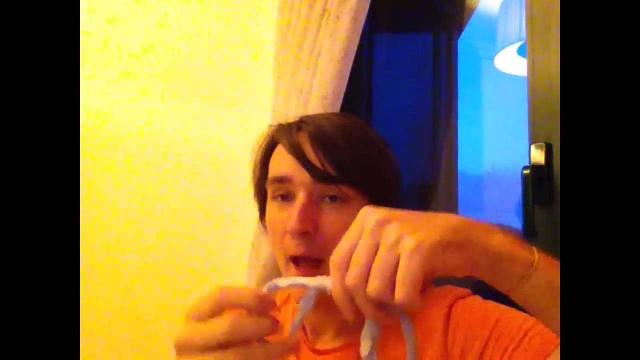 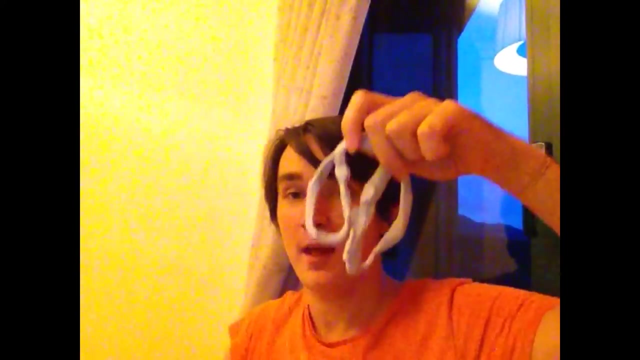 You're not supposed to make any parts of the shape interface of each other that weren't already close to each other. OK, And by doing those operations you can in fact turn those interlocking rings into this shape. They are topologically equivalent, And my problem for you. 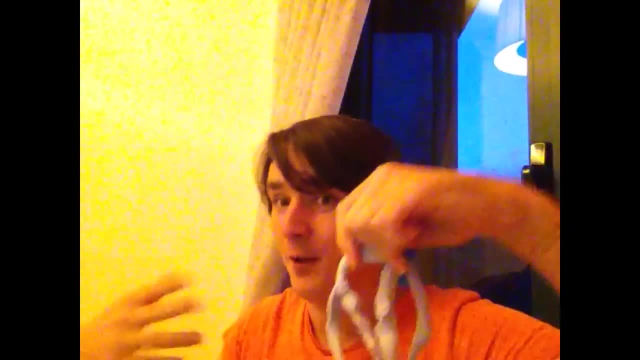 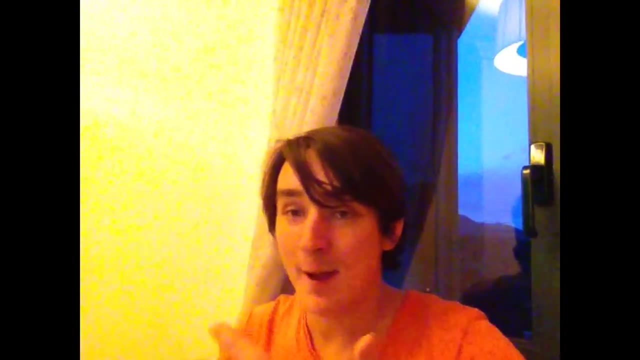 is to show how this is done or draw how this is done. So I think it's a lovely problem. It's the kind of thing that you can try and think about in your head. You can sort of carry it around with you and think about it when you're bored. 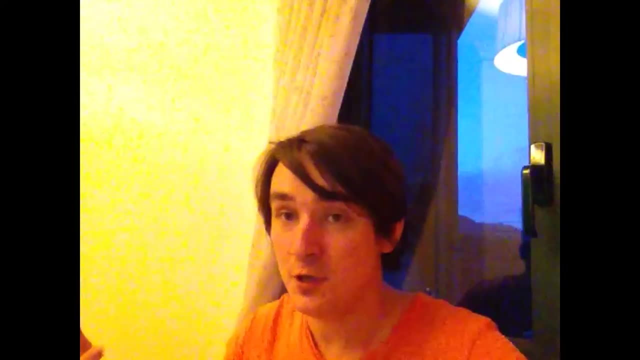 And so I'm going to show you the solution now, But I strongly urge you to stop this video now and basically don't watch the solution. I think it's much better if you try and work out this problem for yourself, Because it's a really fun problem. 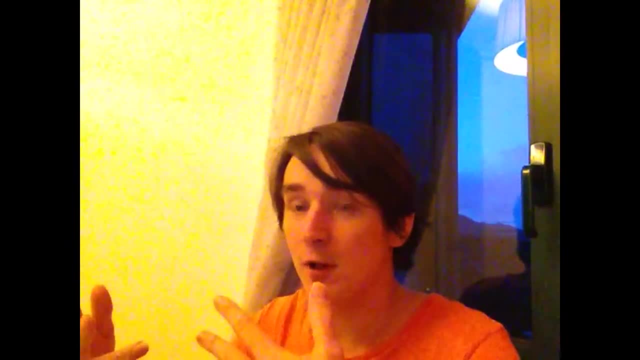 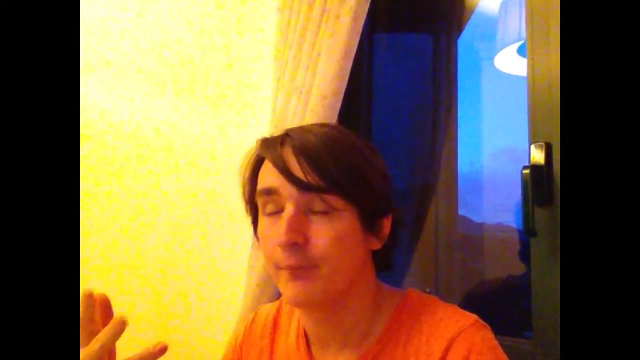 and it will help you to start to get your head around what topology is all about. A good way to do it is you can actually get some blue tack or white tack or plasticine or something like that, So you can really have a go at this problem physically. 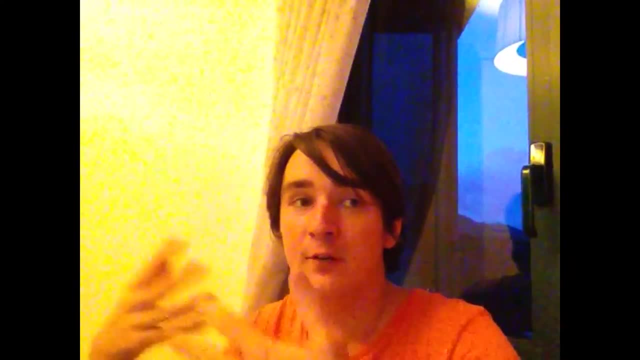 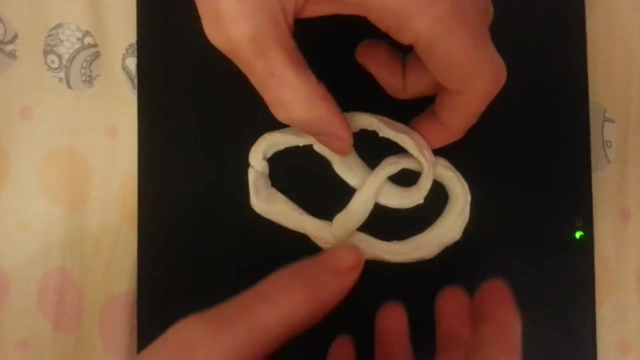 OK, And so next time I'm going to talk more about different kinds of simple surfaces. So I'm going to talk about some surfaces which you've seen before, and maybe a few that you haven't seen before. So here we go. So this is a really simple problem.